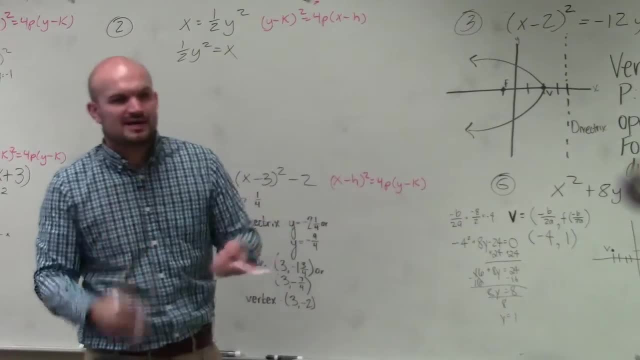 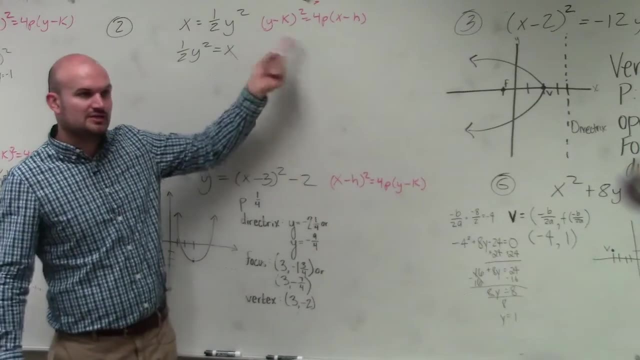 square term on the left-hand side. It doesn't have to be, You could have the square term on either side, But I just wanted to try to look like this equation as much as possible. The next thing I notice is this binomial: here squared is by itself, It's isolated. There's 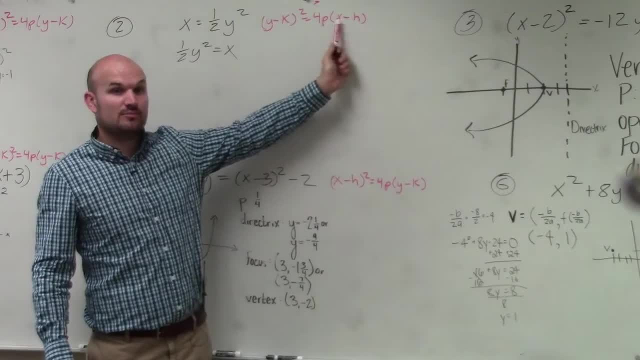 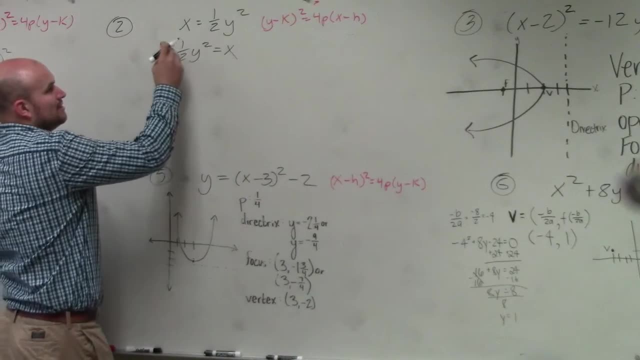 no number that's being multiplied by it. However, the linear binomial has that 4P being multiplied. It has a number being multiplied by it. So what I'm going to do is I'm going to get rid of this 2 over 1.. So I'm going to multiply by 2 on both sides. Then I obtain y squared. 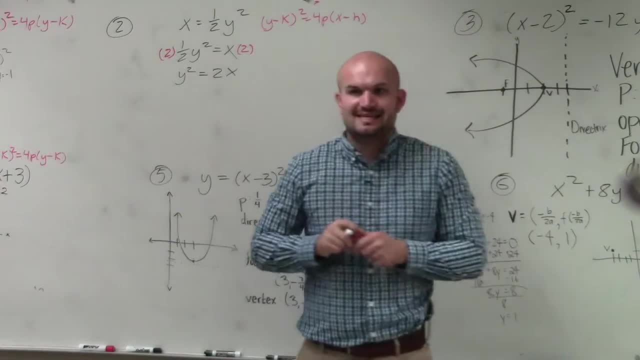 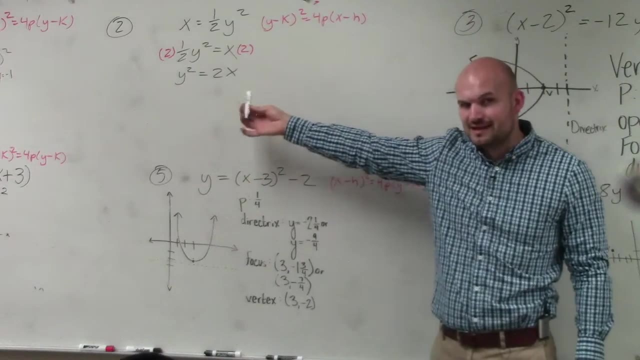 equals 2x. Does everybody see what I have here Now? it's starting to kind of look a little bit similar to this. Now I don't have an h and a k. You can see I'm not subtracting anything. If you wanted to, you could rewrite it like this. You don't have to, But sometimes 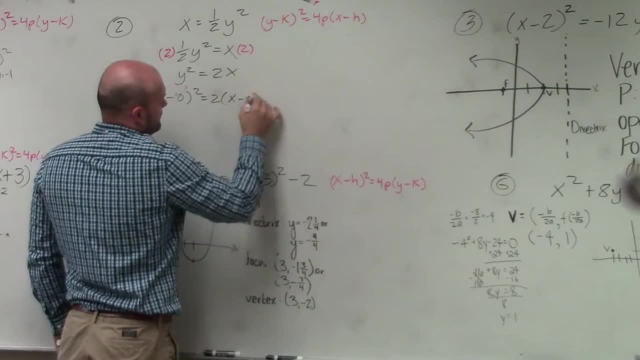 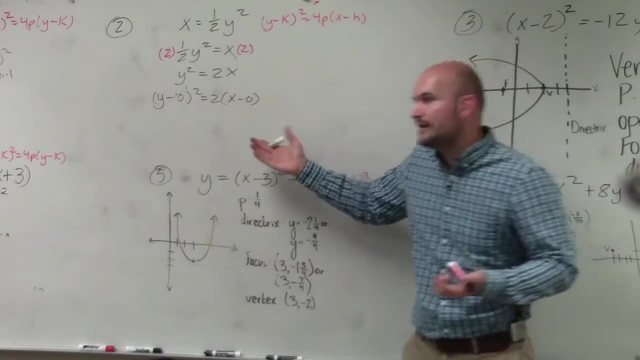 people they're like understand it a little bit. So I'm going to do this, I'm going to do it a little bit better, Like it looking in that format, And I think looking in that format it just kind of makes it easier to understand. oh, OK, h and k, which is the. 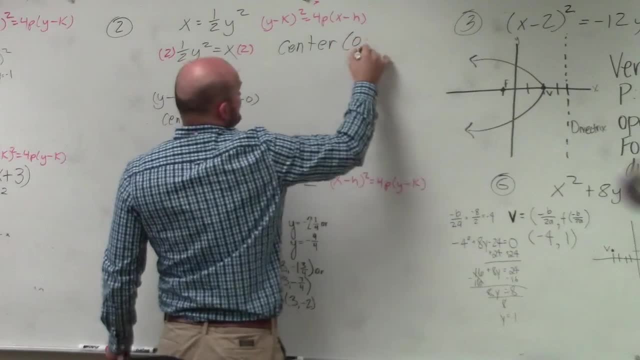 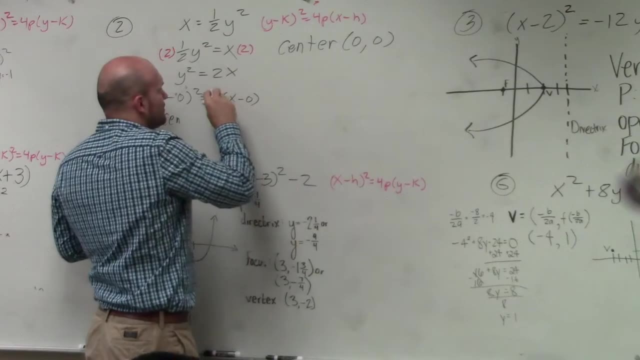 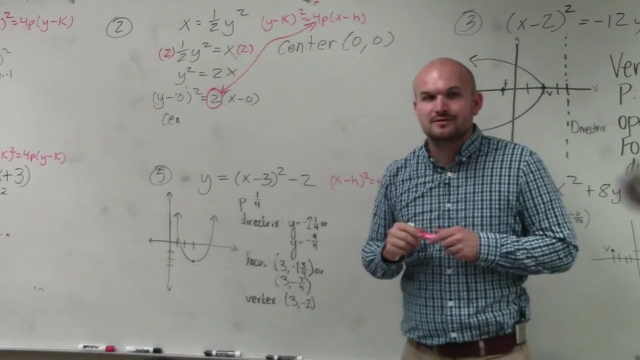 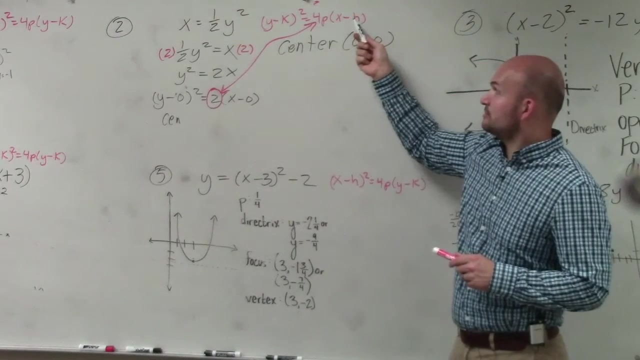 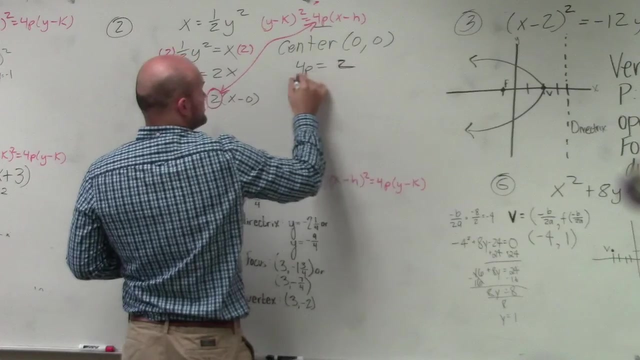 center, which is one of my questions, is 0 comma, 0, right, My 4P is equal to the number 2.. You guys see, Whatever is being multiplied by your linear expression, 4P is being multiplied by your linear expression. So to find P, I do. 4P is equal to 2.. Then I just use some 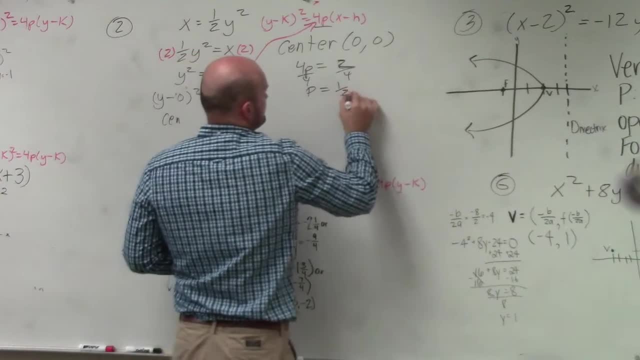 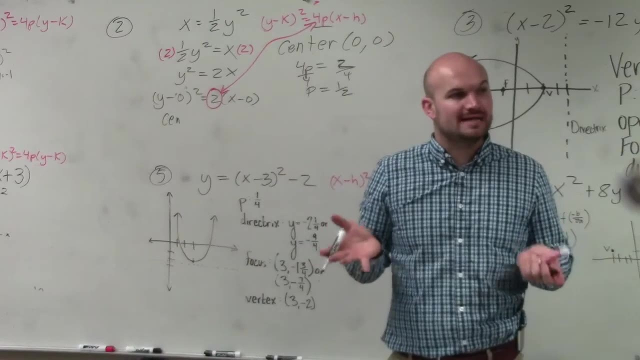 algebra P equals 1 half. Now to find the focus in the directrix: graphing it is a good idea Because I think visually graphing will help you. And this is what I'm saying. I didn't tell you guys step by step what to do. 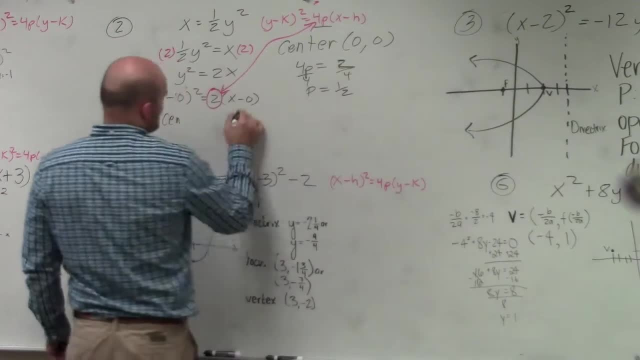 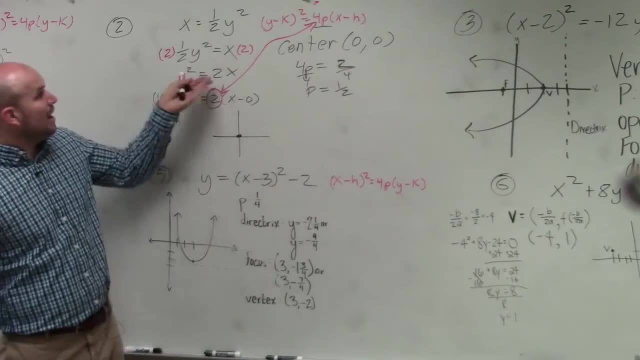 But I want you guys to kind of think about this, All right? Well, let's. I don't know what to do next, Mr McGlogin, So let me graph it and see what happens. The center's here, P, is 1 half. Now x is or, I'm sorry, y is squared. So that means the graph opens left. 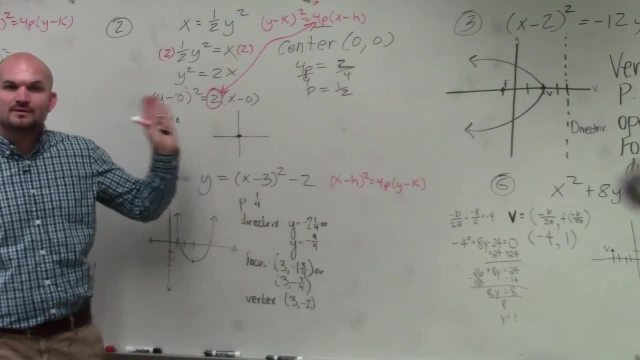 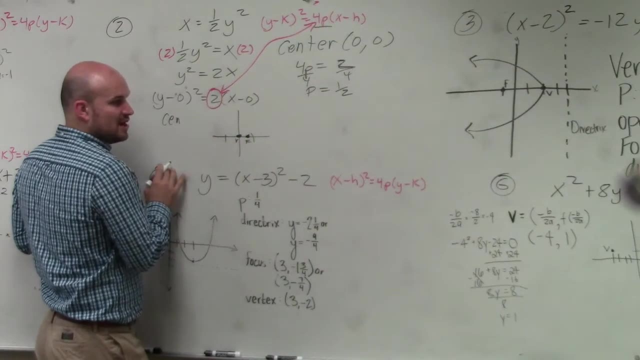 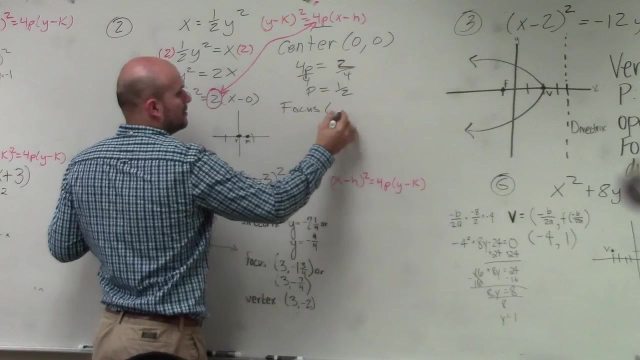 or right, But since P is positive, the graph opens up to the right. So there's my vertex, There's my focus. So if P is only 1 half to the right, what is that coordinate point 0.. 0..